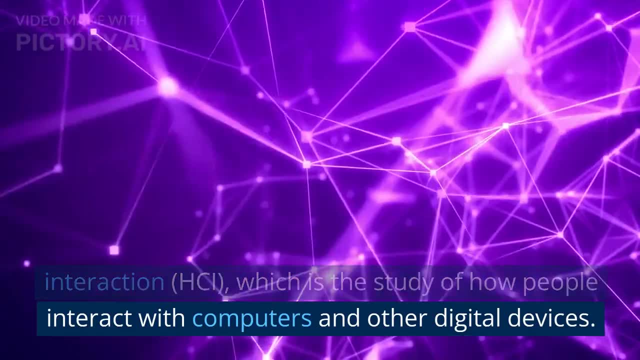 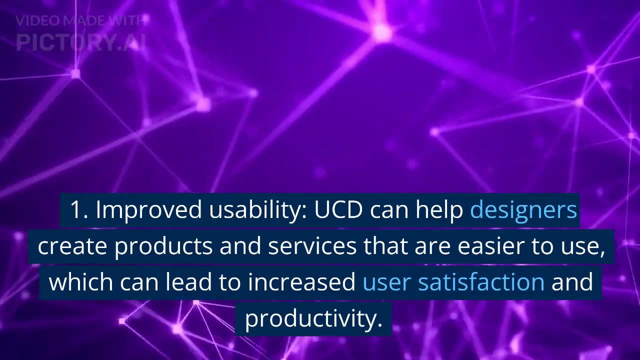 HCI, which is the study of how people interact with computers and other digital devices. Here are some of the benefits of using UCD: 1. Improved Usability: UCD can help designers create products and services that are easier to use, which can lead to increased user satisfaction. 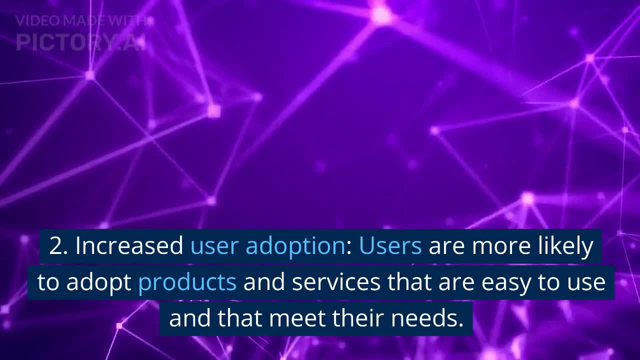 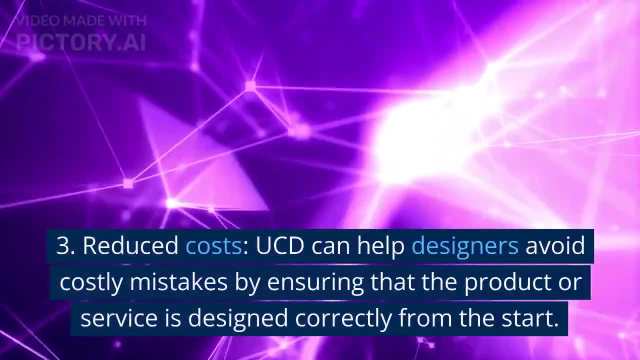 and productivity. 2. Increased User Adoption: Users are more likely to adopt products and services that are easy to use and that meet their needs. 3. Reduced Costs: UCD can help designers avoid costly mistakes by ensuring that the product or service is designed correctly from. 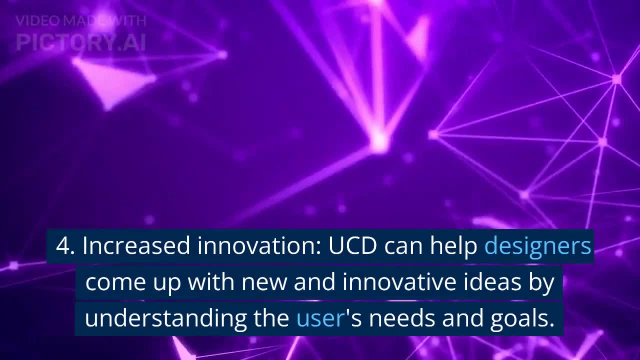 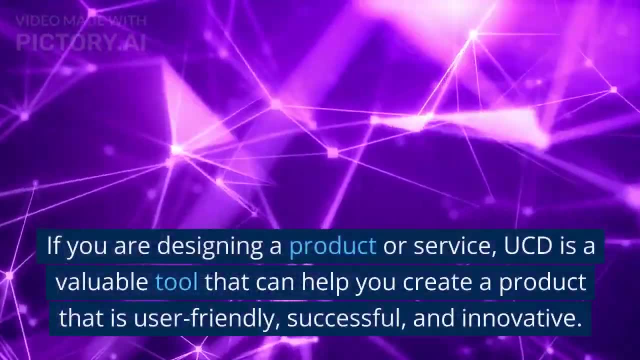 the start. 4. Increased Innovation: UCD can help designers come up with new and innovative ideas. by understanding the needs of their customers, UCD can help designers come up with new and If you are designing a product or service, UCD is a valuable tool that can help you create a. 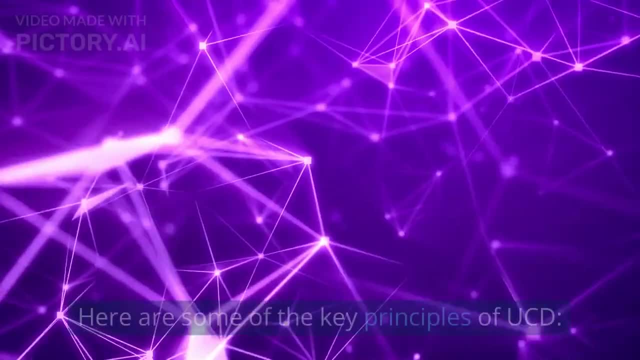 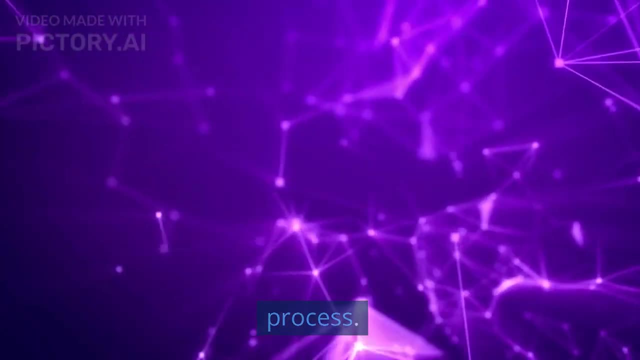 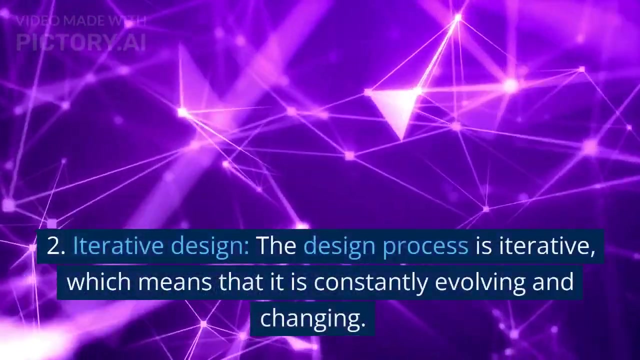 product that is user-friendly, successful and innovative. Here are some of the key principles of UCD: 1. User Focus: The user is the center of the design process. 1. Designers must understand the user's needs, goals and context of use. 2. Iterative Design: The design process is iterative. 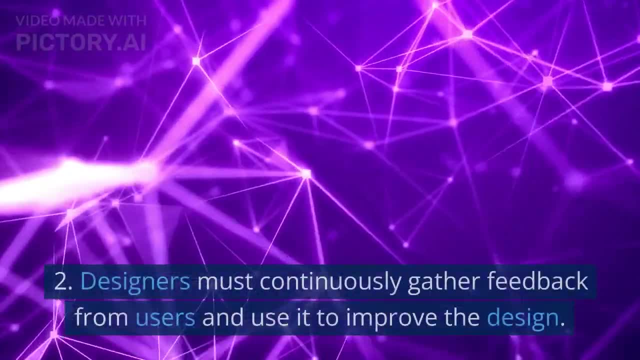 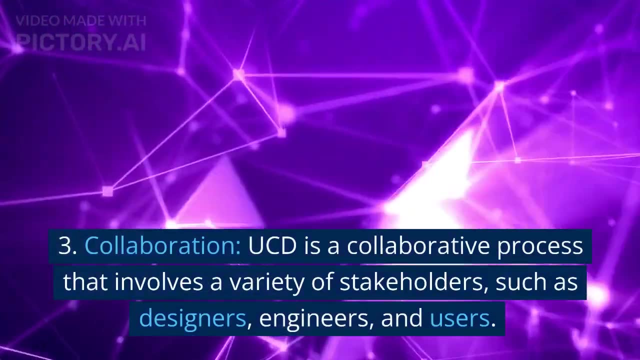 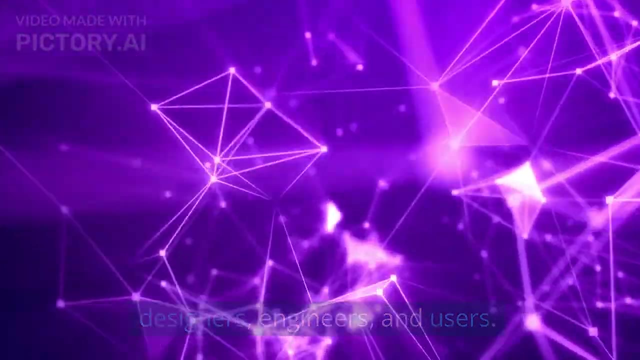 which means that it is constantly evolving and changing. 2. Designers must continuously gather feedback from users and use it to improve the design. 3. Collaboration: UCD is a collaborative process that involves a variety of stakeholders, such as designers, engineers and users. 4. Prototyping: Prototyping is a valuable 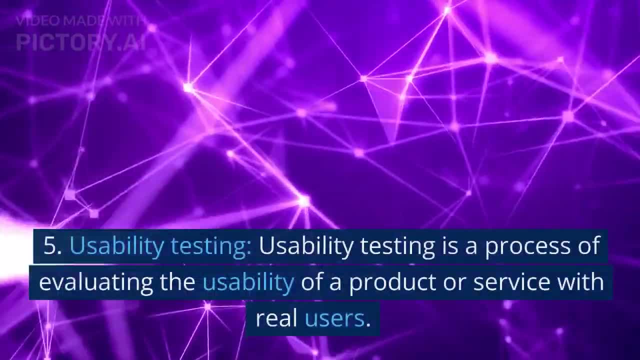 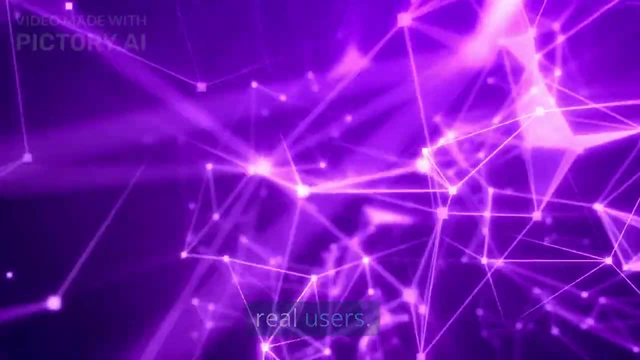 tool that can be used to test and refine designs. 5. Usability Testing: Usability testing is a process of evaluating the usability of a product or service with real users. UCD is a complex and challenging process, but it is a valuable tool that can help designers. 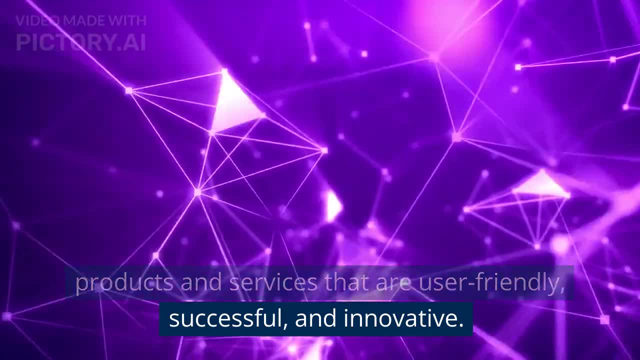 create products and services that are user-friendly, successful and innovative.